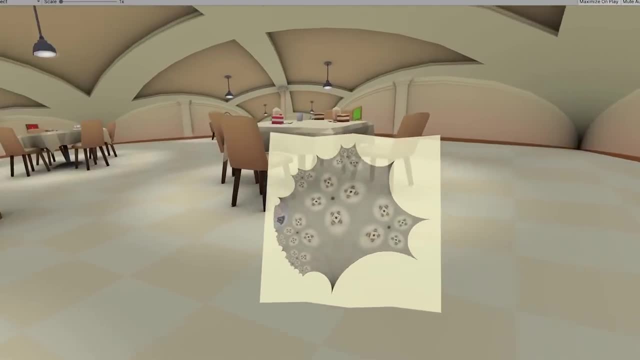 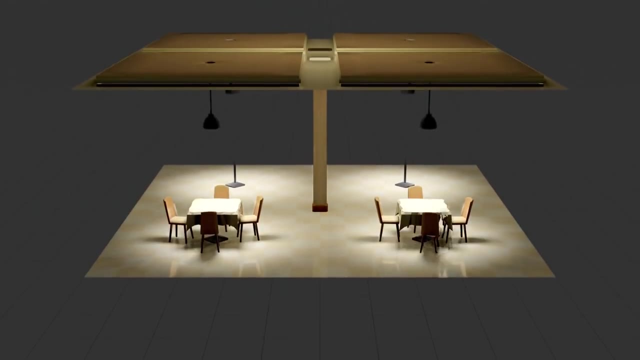 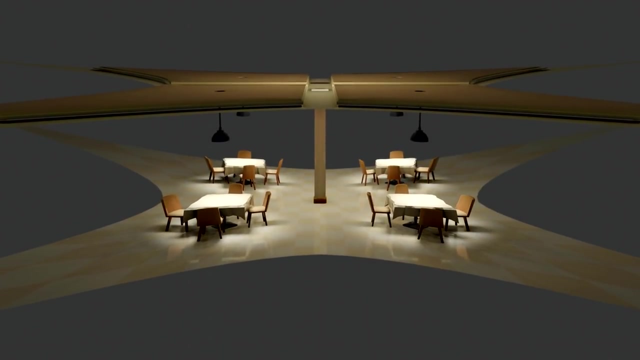 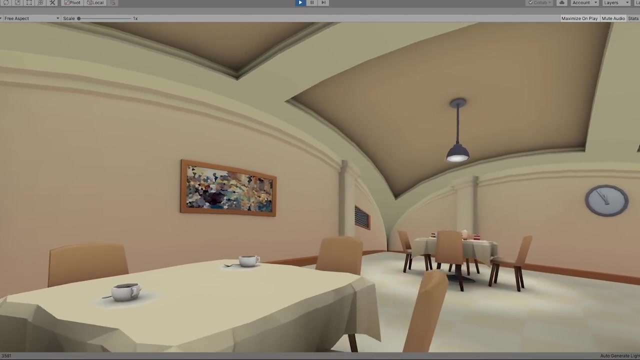 The most noticeable one is probably the horizontal distortion. When we take an object that's modeled in Euclidean space and project it to hyperbolic or spherical space, even though the lines stay straight, the angles and sizes get distorted, And so in a hyperbolic space, the closer an object is to the corner, the more stretched it becomes. 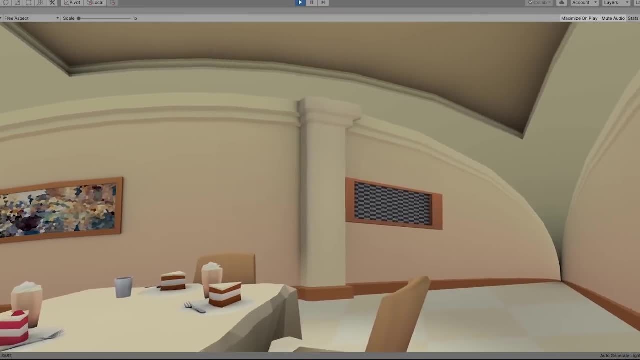 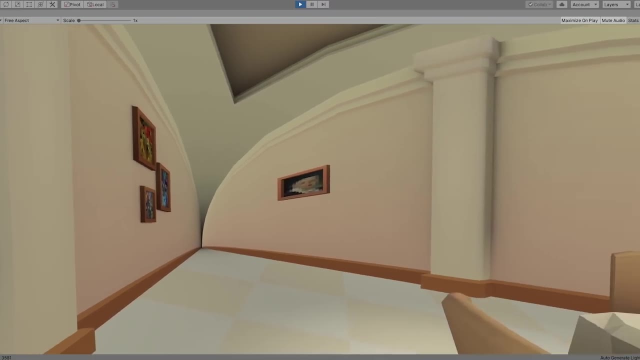 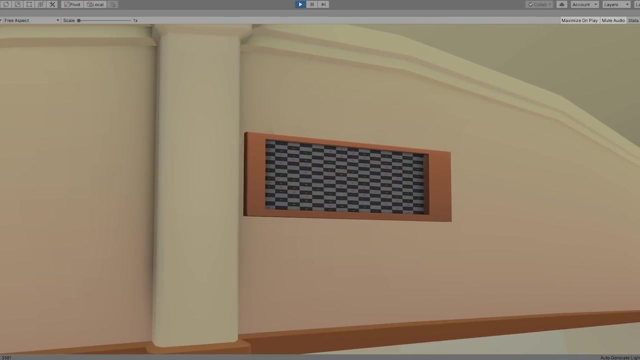 So let's say we want to make these paintings look right in the game. The closer they are to the corner of the tile, the more we have to make it squished to compensate for that distortion. And besides horizontal distortion there's also vertical distortion. 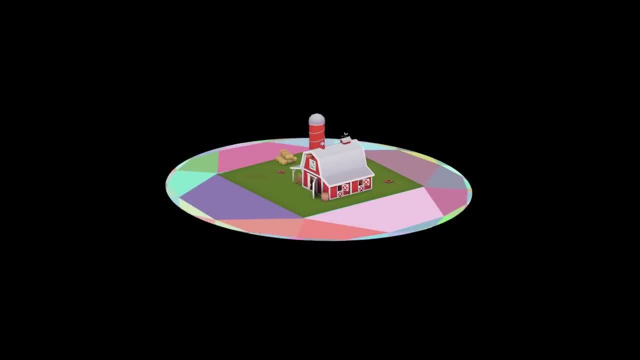 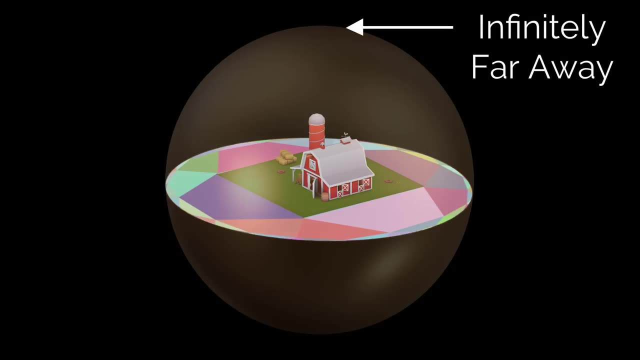 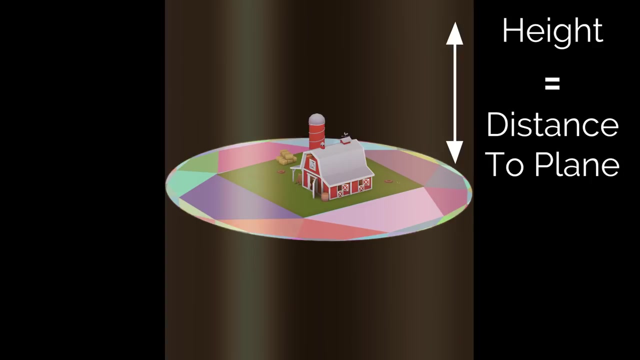 And due to mapping from Euclidean space to hyperbolic, it means there's a height limit where things get mapped to infinity, And this invisible limit can make modeling difficult. so, to make things easier, Hyperbolica remaps height to match the actual hyperbolic distance. 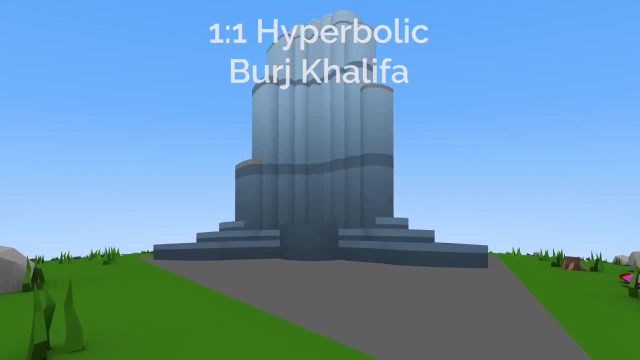 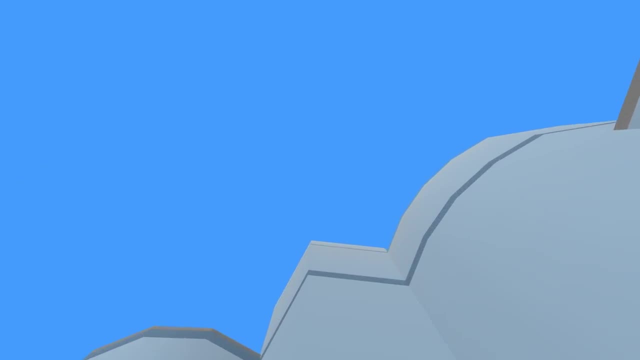 And doing this makes it easy to build saw objects without worrying about limits, but it also means heights get distorted in a different way. This is a very advanced piece that can be easily integrated into a simple chart, even if you've never done a field chart before. 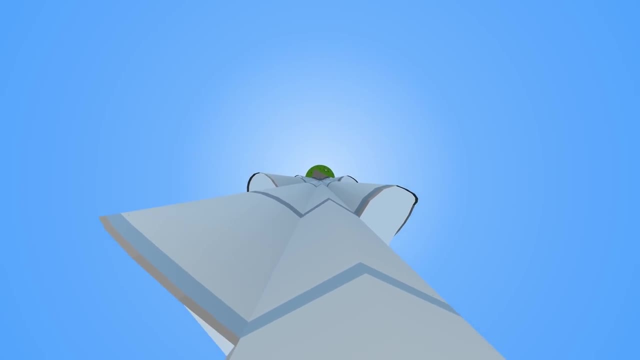 The first thing we do is make a new path, one that's a little more linear than a horizontal one. The first tree on the graph shows what the depth will be, ie the height of the other. The third tree shows the depth of the other and the depth of the further one. 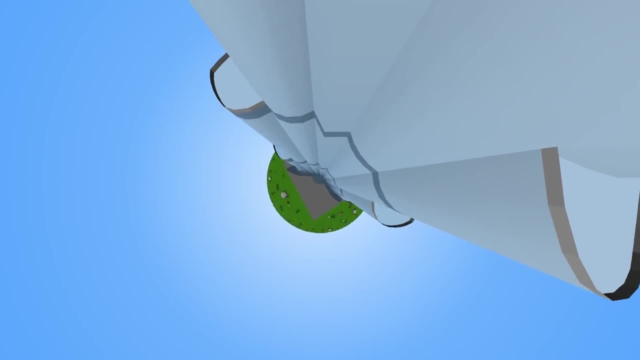 The fourth tree shows the depth of the lizard. The fifth tree shows the depth of the others. The last one shows why and how different all these elements are. This is what many people think. When you're looking at the map, the different projections mean that even the straight lines 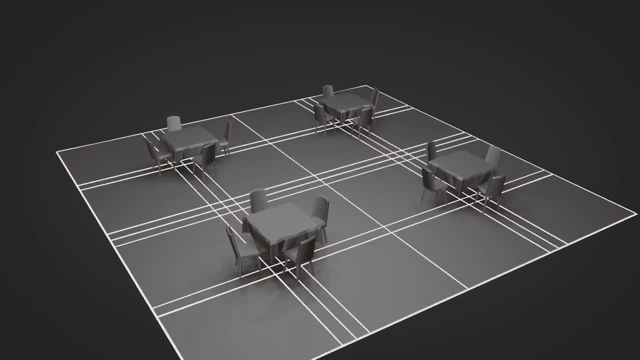 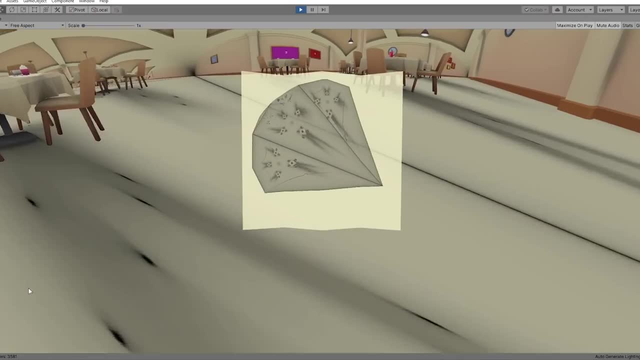 have to bend, and because of that we have to add this particular subdivision pattern. In this example, the corners of this tile stretch all the way to infinity, and if we had no subdivisions on the floor, the outline would look very choppy. 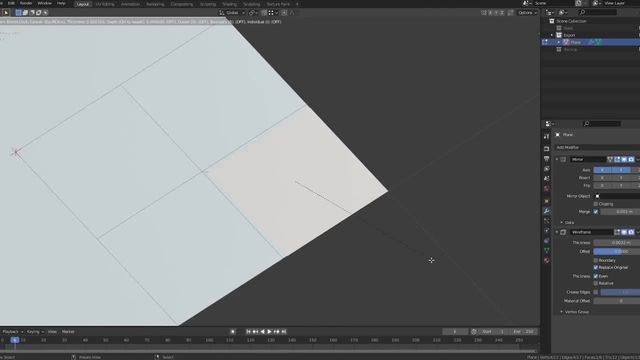 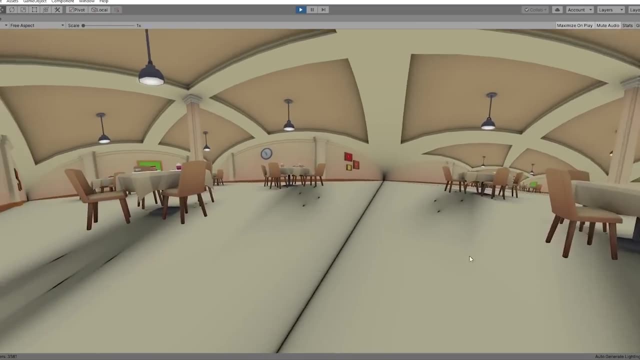 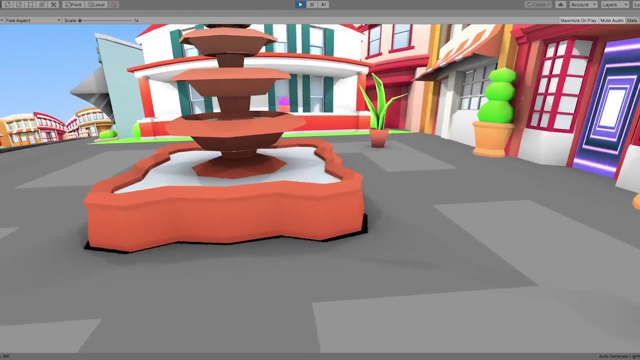 So to get smooth curves, the floor gets a cut halfway to the corner, then a quarter, then an eighth, and so on. Another problem that you might notice is that the shadows don't always lighten up with the objects that cast them, And this is because shadows and image occlusion are baked into each section. 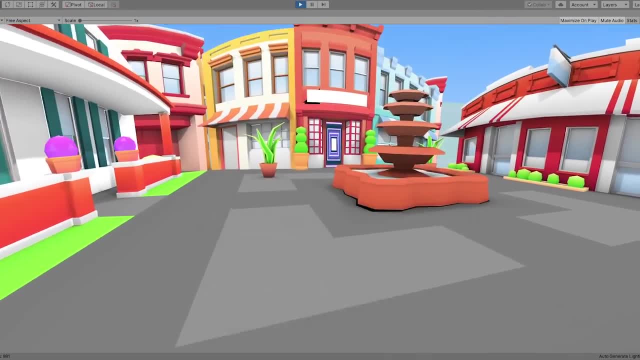 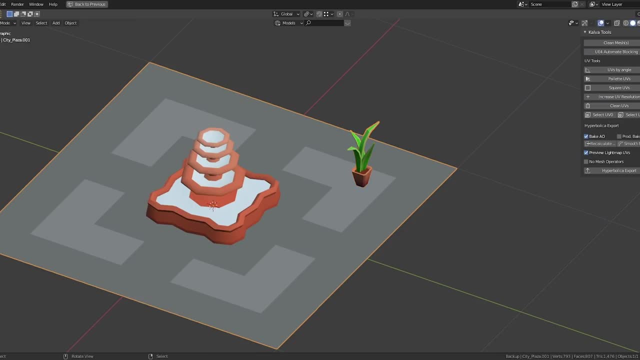 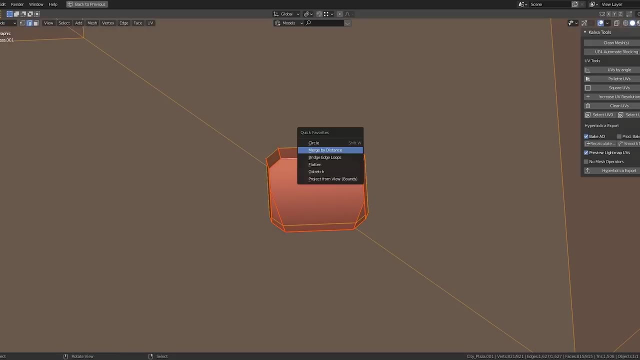 But it doesn't get interpolated perfectly, since only vertices get the right transformations, And subdivision can help, but it's not the best solution. The best one is to remove any self-intersections in the geometry. Every edge needs to be separated, Every object needs to be shared with neighboring triangles and can't just sit on top of them. 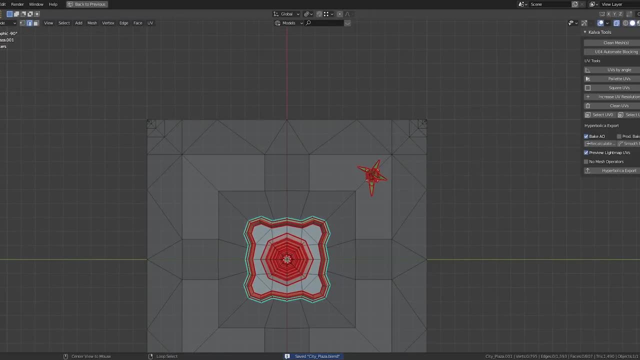 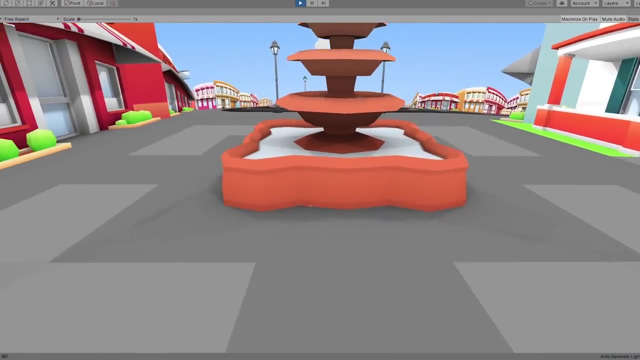 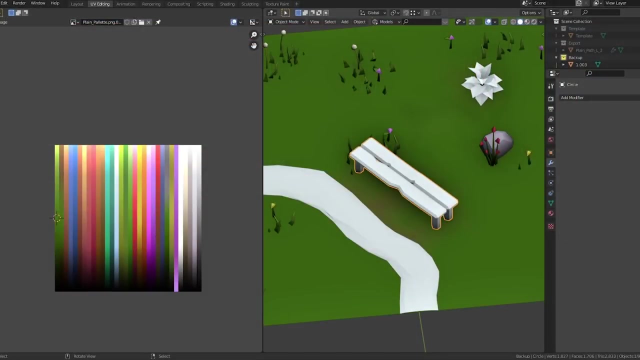 or intersect, which is something that is quite common in 3D modeling. After we make the geometry, it's finally time to give it some color, And traditionally each object has several materials with different textures that give it color. But in our case, we had to think about a lighter approach. 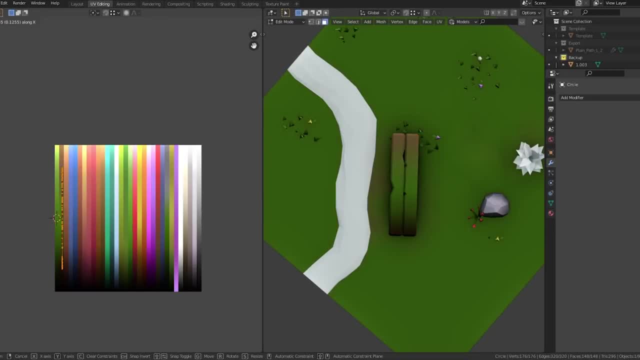 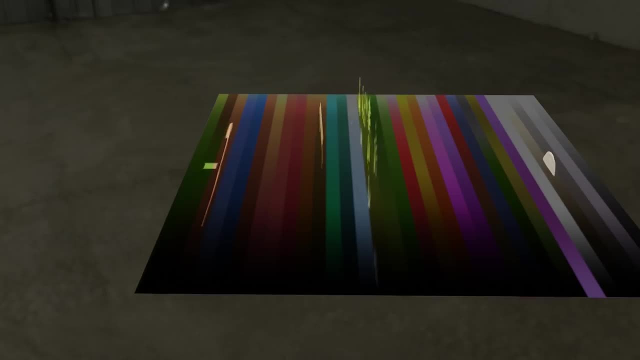 And we ended up making so. most objects share a single small texture. The tile UVs are projected from a plane which is then infinitely squished in the horizontal axis, making it so you can control which gradient you want to pick and how big it's gonna be. 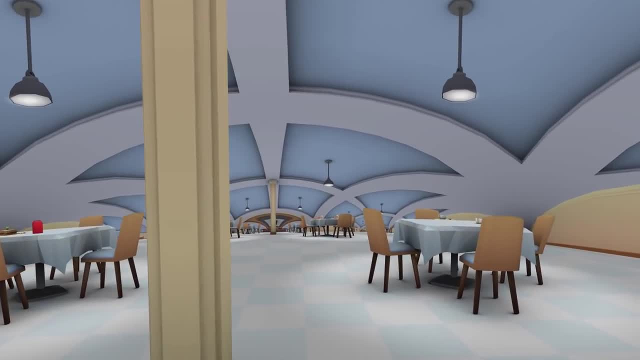 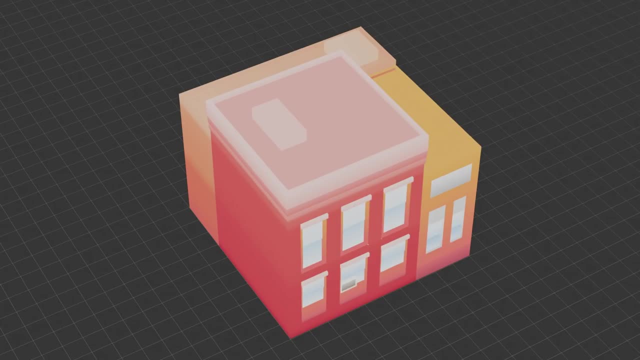 And, as a bonus, if we wanna change the color theme of a scene, any change to the palette is carried through all of the tiles, making it really quick to iterate. Each object carries two UV channels. The first one uses the palette to define its colors. 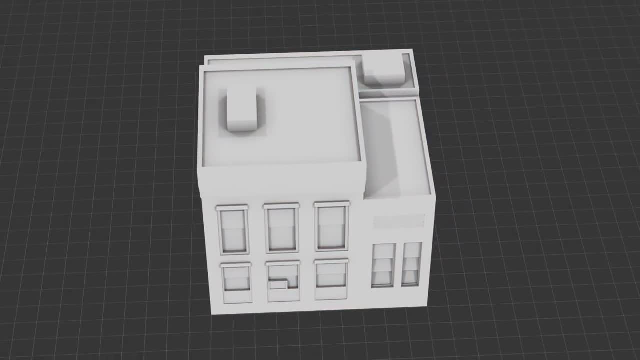 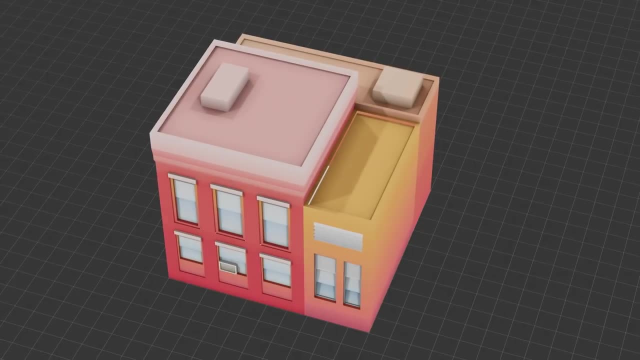 And the latter uses the lightmap with traditional UVs to define the shadows and image occlusion. In the end, they both overlap in unity to give the final shaded look. Adopting a low-poly art style allows us for a go for these optimizations, which are especially 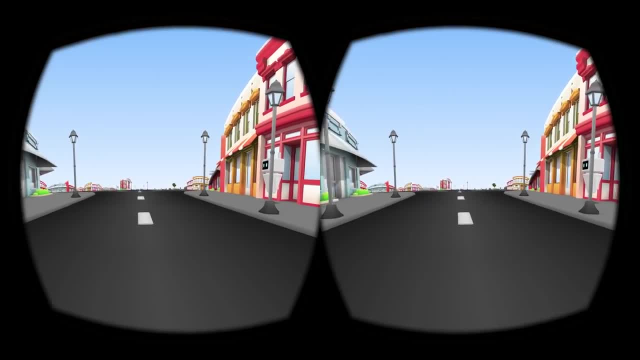 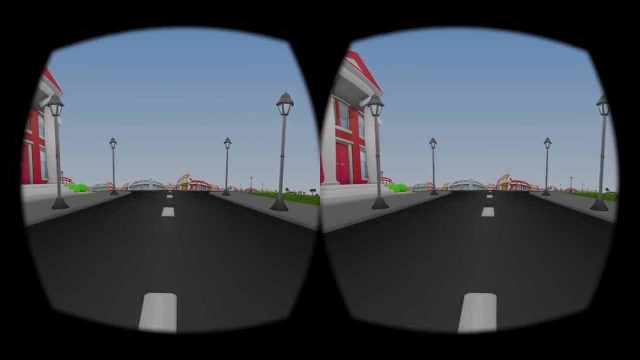 important when you keep in mind Hyperbolica is also going to run in VR And it also gets the point across without being too time-consuming. so that's why we decided not to go with the PBR workflow for now. We're making all of the assets now. 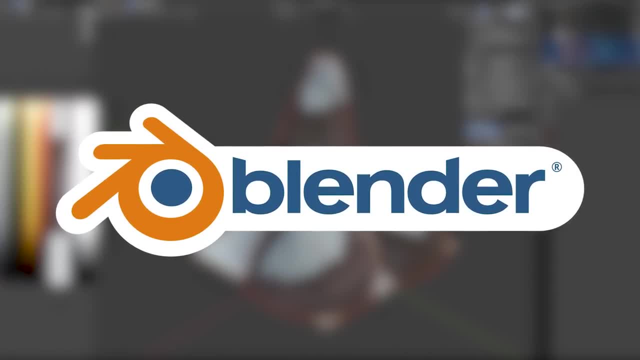 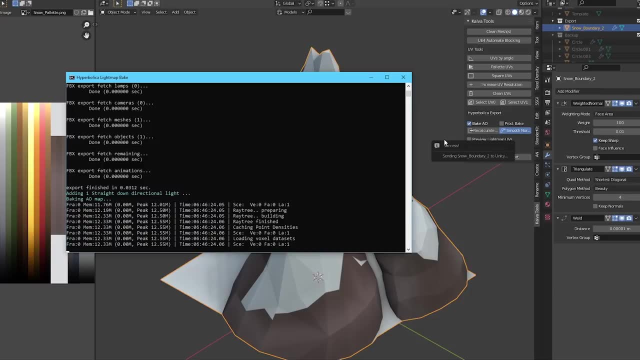 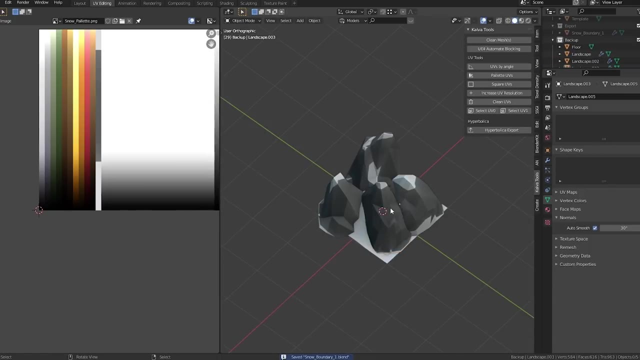 We're going to add a little bit of color. We're going to add some assets in Blender, an amazing 3D software that is completely free, along with some custom Bison scripts we made to help us automate most of our workflow And, as you can see, most things are really uncommon to anything you learn about 3D modeling.